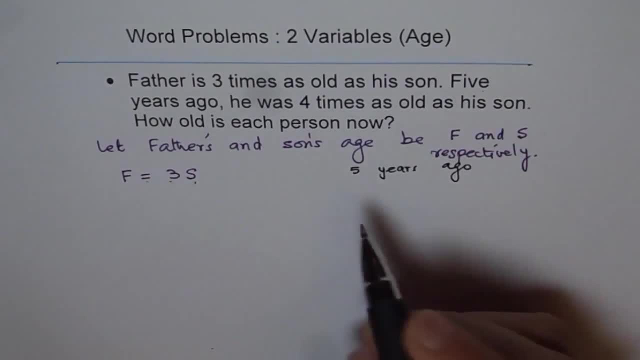 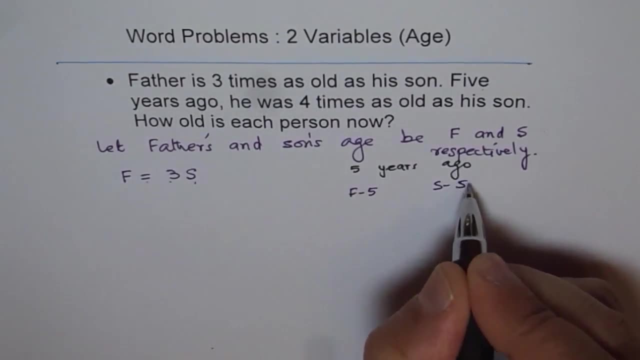 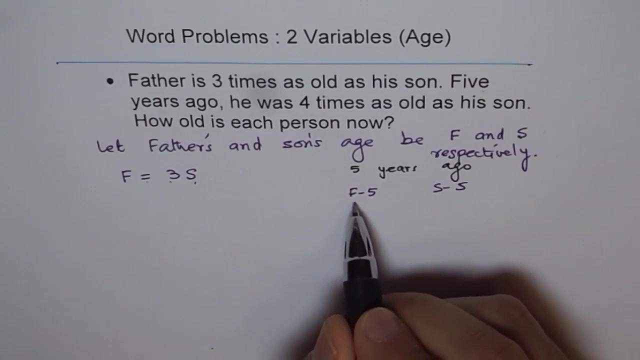 age is F and S. what was the age five years ago? It was five less right. So the age was F minus five and S minus five. I hope you appreciate that part. This is what you have to work out. Five years ago, father's age was F minus five and son's age was S minus five. Now read again. 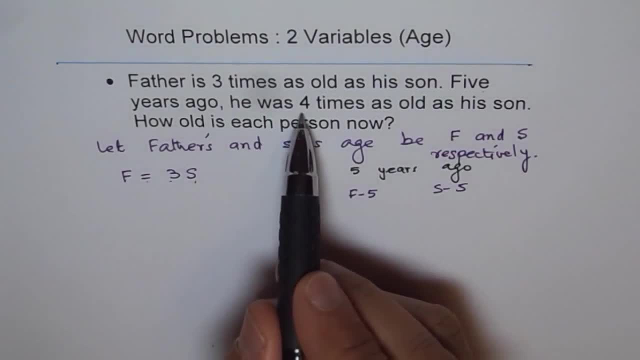 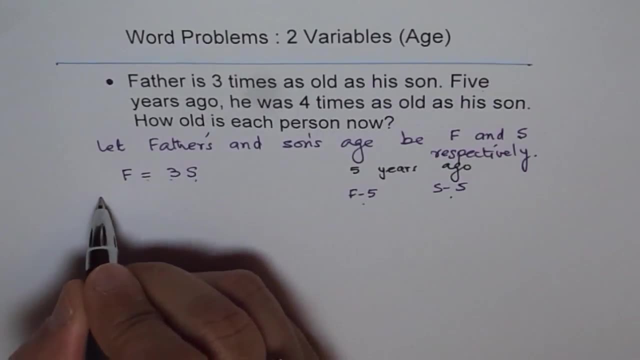 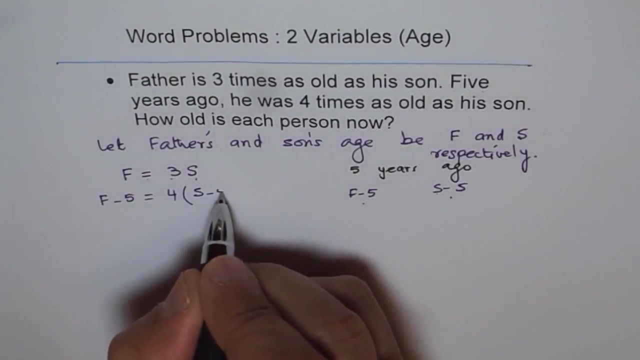 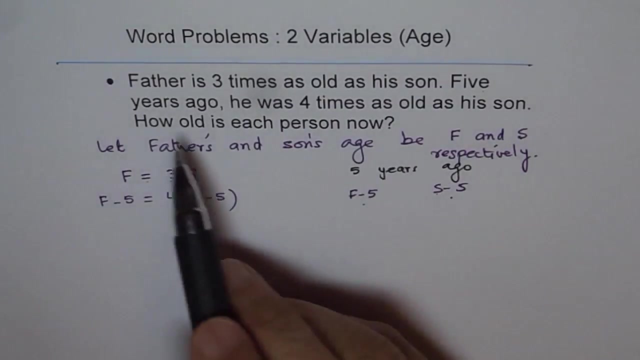 Five years ago he was four times as old as his son. That means this was four times this. So we'll write another equation, which is F minus five equals to four times S minus five. Do you understand that? Have a good look, Rewind and go through it once again. Five years ago he was so F minus. 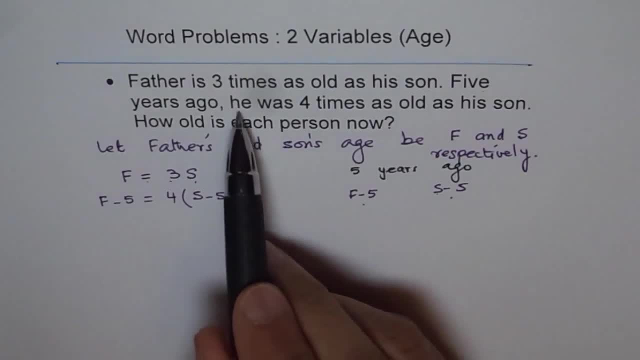 five is five years ago, 5 years younger also, right, He was 4 times as old as his son, 4 times son's age. Son was also 5 years younger 5 years ago. So we get the second equation. So that is how. 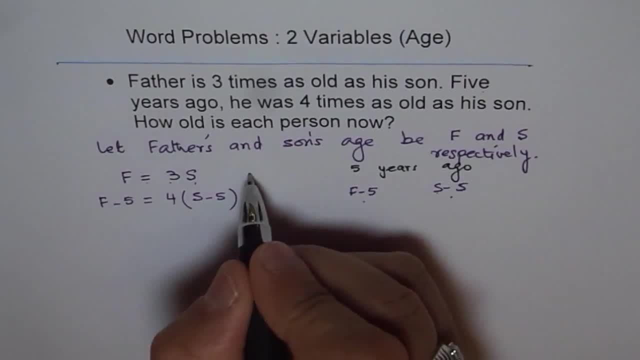 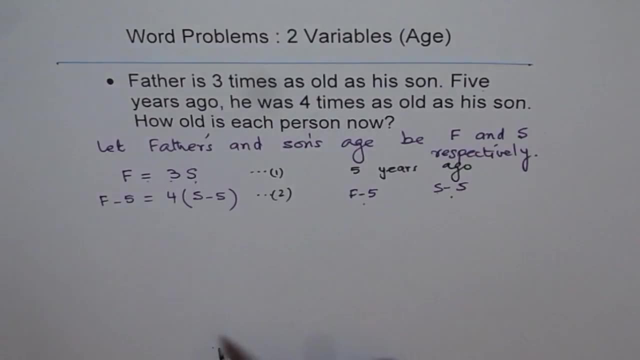 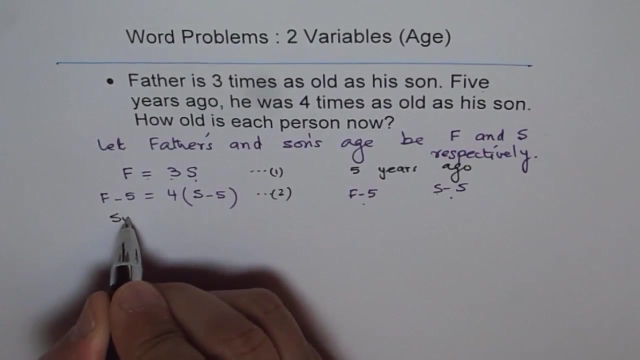 you get two equations. Now, once you have two variables and two equations, you can solve for the variables. Let's number these equations and decide what method to use. Since we know f is equal to 3s, we can use substitution, So substitution is a method of choice here. 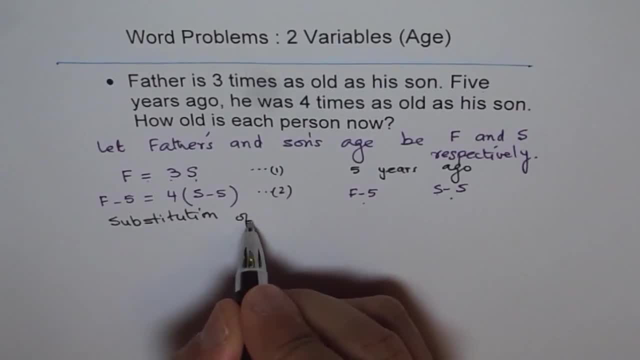 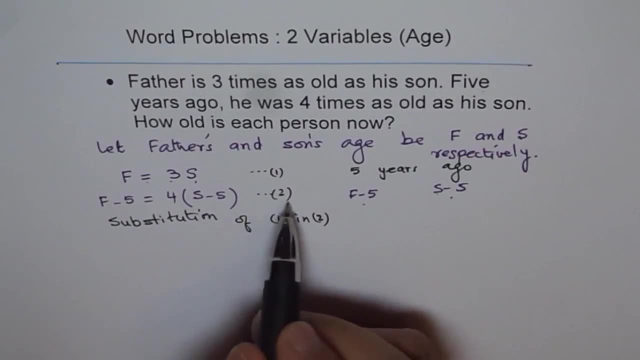 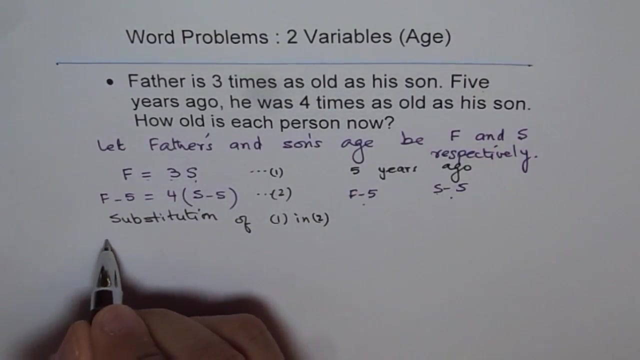 So what will we substitute? So this is a substitution of 1 in 2. That means the value of f from equation 1 will be substituted in equation 2. to solve further: So f is equal to 3s, So we will write instead of f 3s. So we will say 3s minus 5 is equal to 3s, So we will. 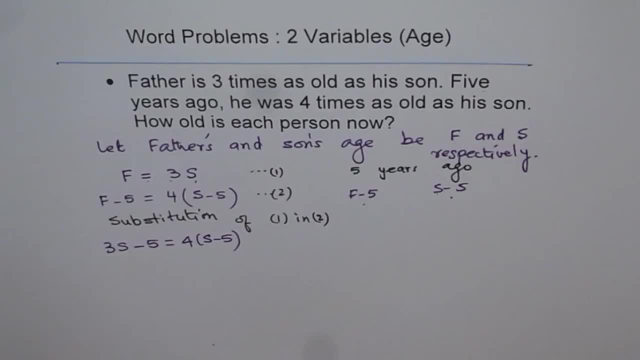 write: 3s minus 5 is equal to 4 times s minus 5.. Now you see, we have equation in one variable, So you can solve for s. Let's rearrange: 3s minus 5 is equal to: let's multiply First.